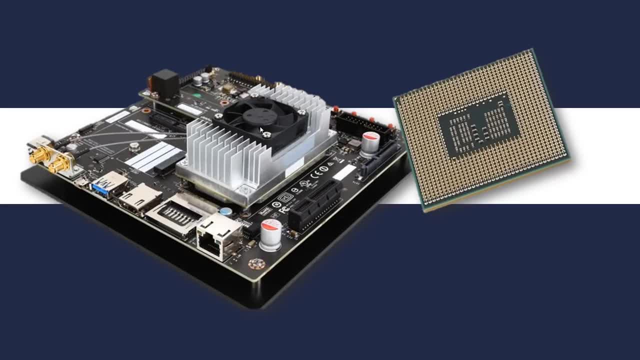 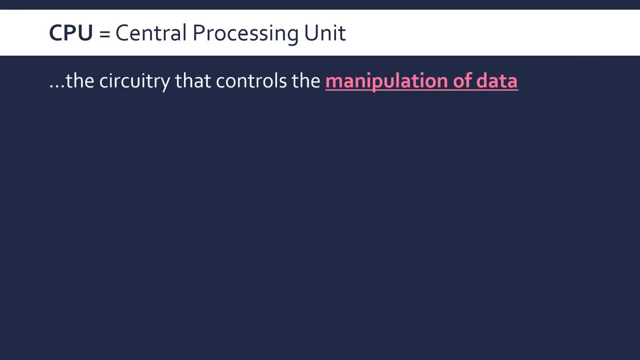 So this is where you'd find it, actually as the hardware device on the computer, But we'll be looking at it from a more theoretical point of view in this video. So it stands for Central Processing Unit, and it's the hardware that controls the manipulation of data, processes data- that's what it does. 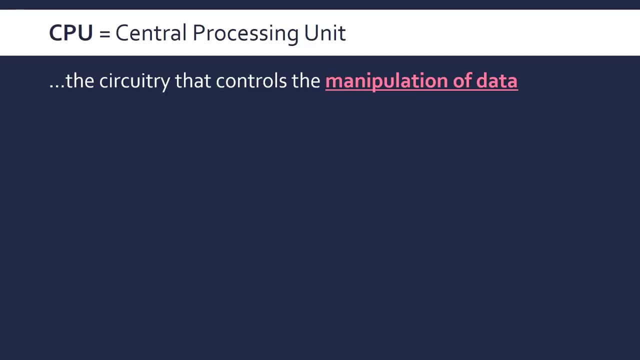 And it's worth pointing out that in a computer there are potentially several processors. Not only can you have multi-core CPUs, where you have kind of like several CPUs within a CPU, if that makes sense. We'll look at that a bit later. 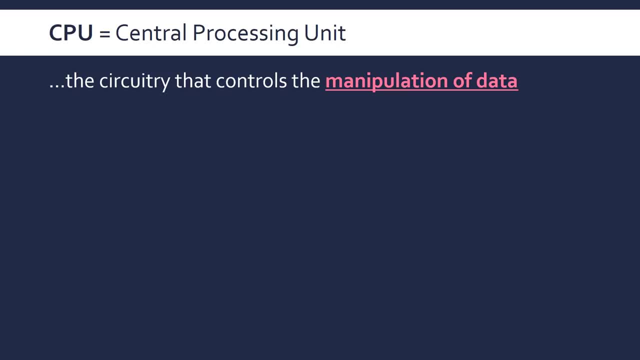 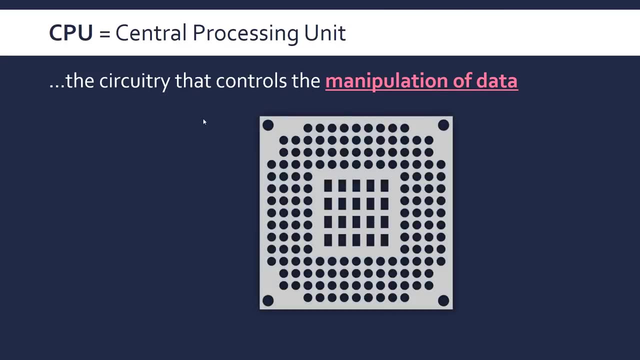 But you also have processors in things like graphics cards and sound cards. So processors are kind of like a drive. They're not really a general term, but it is used interchangeably with CPU. Just bear that in mind. But to start off, let's just break it down into three components. 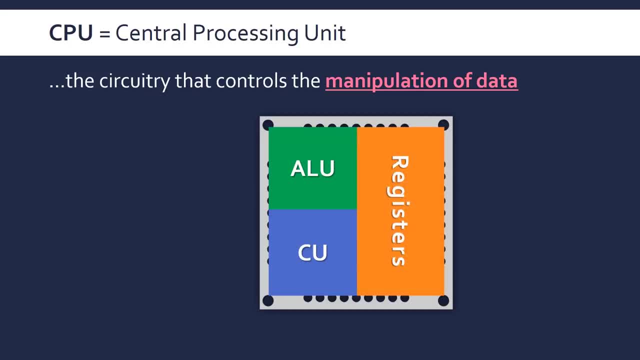 The ALU, the control unit, the CU and the register unit. So, firstly, the CPU isn't obviously this simplified, but firstly, the ALU is actually what does the processing that actually carries out the instructions. This is the arithmetic logic unit. 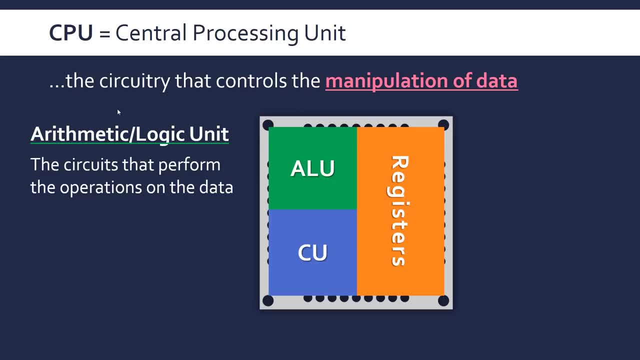 It's written with a forward slash for some reason. I can't say I know why, but it is So. ALU- arithmetic logic unit, And this actually performs the operation. So ALU is the CPU. So ALU is the CPU. 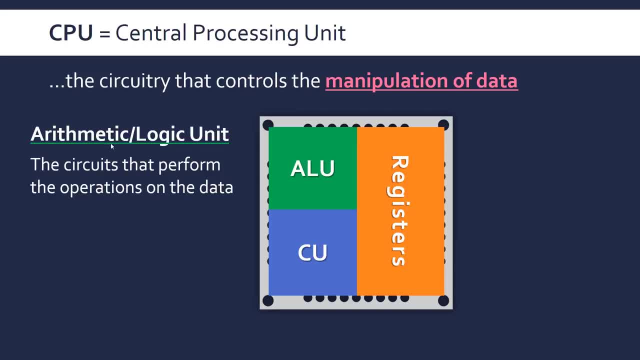 And this actually performs the operation. So it performs the arithmetic operations like addition, multiplication, division and so on, And the logic ones, like I mean basically evaluating something to false or true, the two Boolean values. So this is what actually does kind of the hard work. 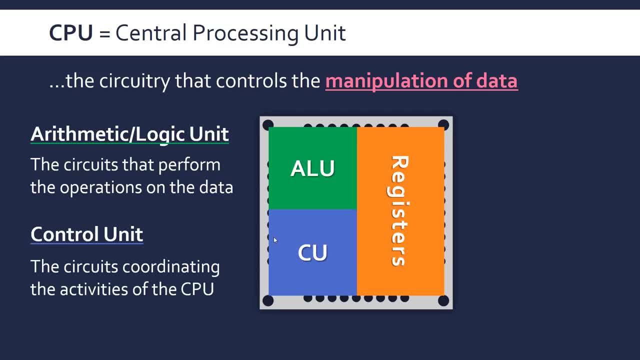 But it's overseen by the control unit which actually coordinates the CPU, And because the CPU is kind of what is controlling the whole computer, it's what's doing all the computer's processing, apart from these potential graphics cards, sound card processors, which is doing a very specific task. 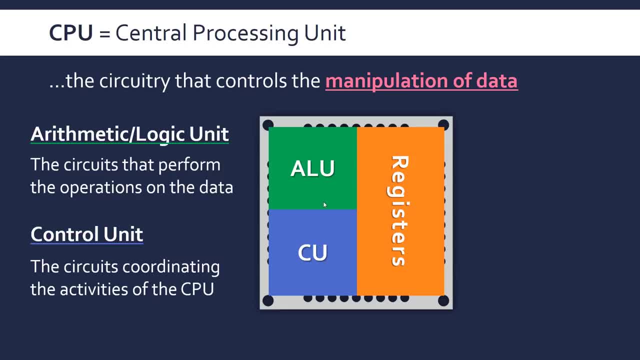 But generally. But generally it's controlling the whole computer. You wouldn't be watching this video if the CPU wasn't working in your device And the control unit actually kind of warms up the circuitry. it decodes the instructions, actually deals with the data transfers and so on. 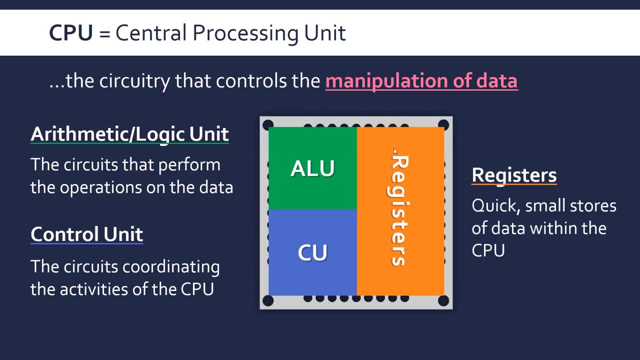 And the registers are small, quick source data. You might have say I don't know 32 on your CPU And some of them are used for programmers. Some are used for the fetch execute cycle, which we'll cover later. 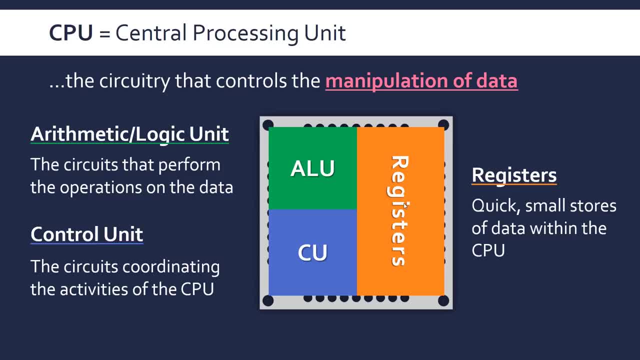 They're very quick, very small. They're actually on the chip and they're mostly there for efficiency, because it's very slow comparatively to have to keep going back and forth between memory. They're used kind of like a temporary storage on the CPU and they're used in its operation as well. 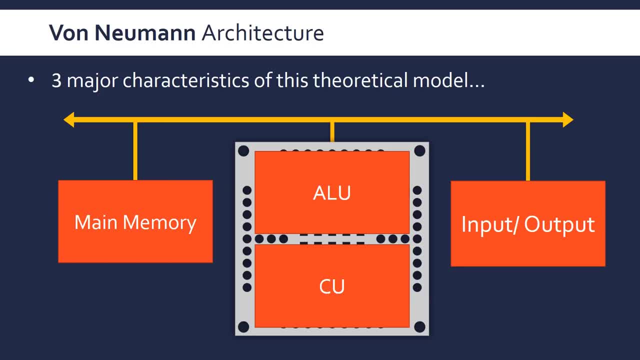 So I wanted to talk about Von Neumann architecture briefly, and this is a term for essentially what we've just looked at. It falls under this category, and all the hardware we're looking at, all the modern computers, fall under this category of Von Neumann architecture. 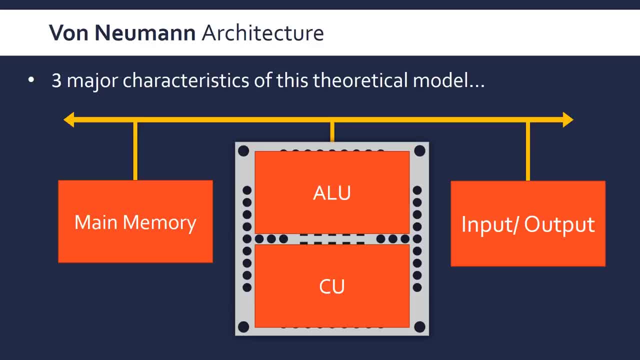 And this is often a point of confusion, Because it's not really taught, Because it's so ubiquitous, because everything essentially is based on this architecture. it means the teachers don't really explicitly say it's Von Neumann architecture. People often get confused because they see this term and they're like I've never heard of this before. 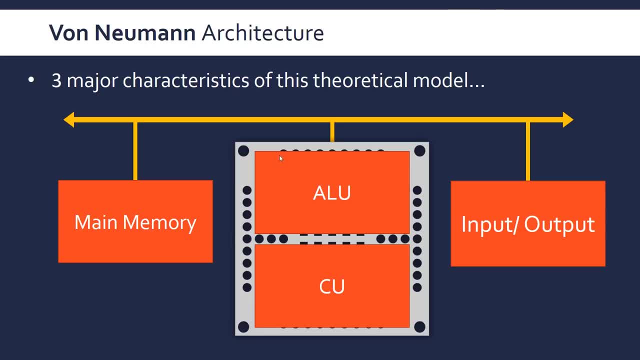 And actually it's what we've learned all along. So you know, you don't really have to know about the other architecture, the other models available. This is going back to 1945.. But essentially it says that we can break our systems down into four components: the main memory, or just memory, which is where the registers in this. 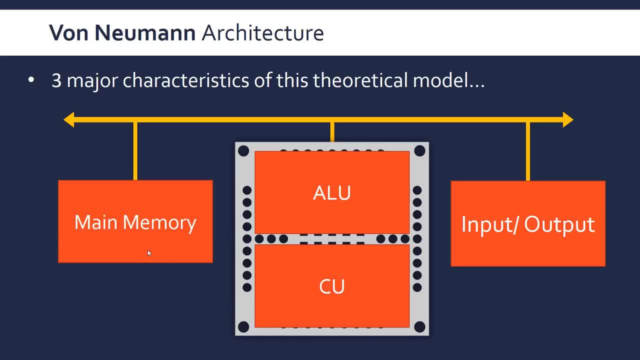 Kind of model would fit in, and we'll talk about memory a lot more in the hardware videos. but also we've got ALU, we've got a control unit- This is the processing unit of this theoretical system- and we've also got input output devices. 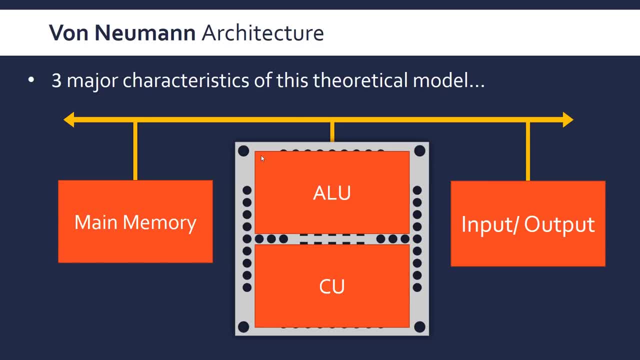 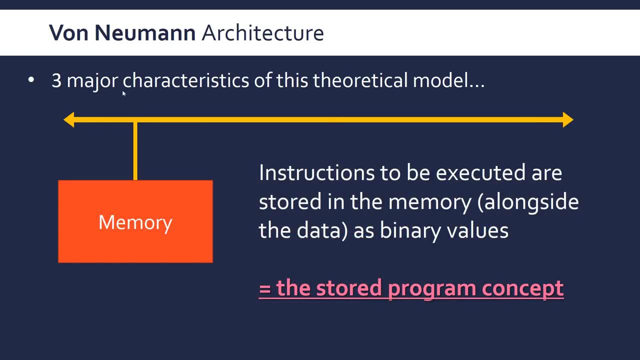 And again this is going back to 1945. So if you can imagine the processes and the computers as a whole back then, this is very simplistic. But this does also mean a second major characteristic of this is that the instructions are executed. the instructions that are executed are stored alongside the. 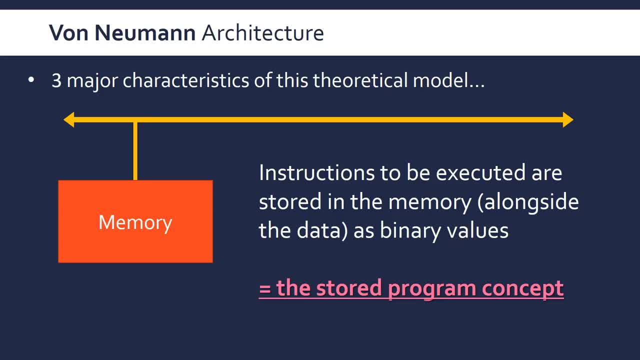 data in the memory, So everything is stored in the memory alongside each other in binary, as we would have talked about another point of the course, And this concept, the fact that the data and the instructions are stored together, is the stored program concept. 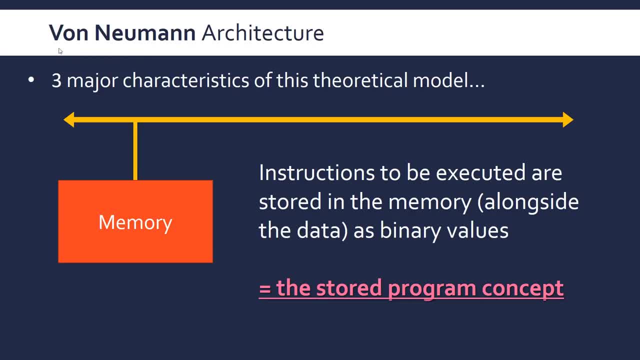 And again, this is often attributed to Von Neumann, perhaps unfairly, to the people who actually did it, because I think he was just anyway, he was very famous. But this contrasts with another model which isn't really used in modern computers, and this would be the Harvard model. 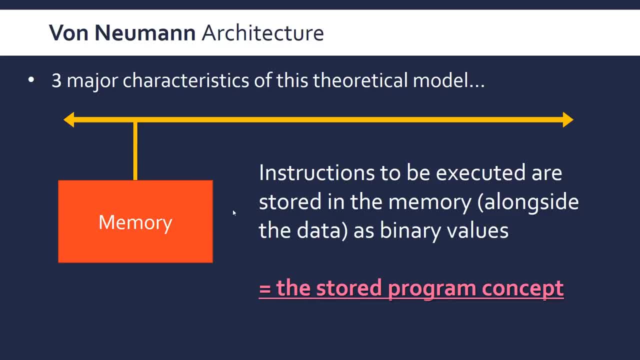 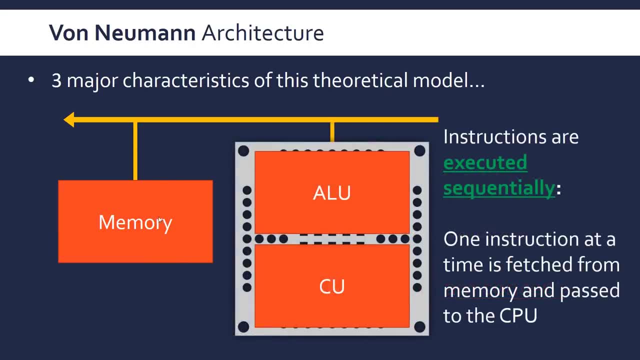 And in the Harvard model there's basically two different, two different memories: one for the instructions and one for the data. but we don't use that, so we're not going to worry about that too much. In the Von Neumann model, architecture instructions are executed sequentially and this is how. 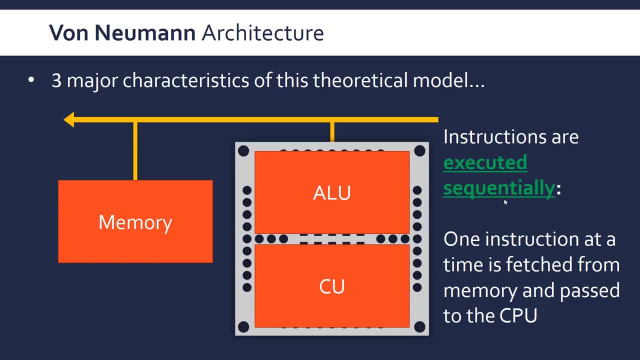 it works in our computers so one instruction at a time is fetched from the memory and passed to the CPU. and this means that even if your CPU is absolutely rapid and it's very, very fast, if the connection between memory and the CPU in this bus, in this wire, if it's very slow, you get a bottleneck, which is 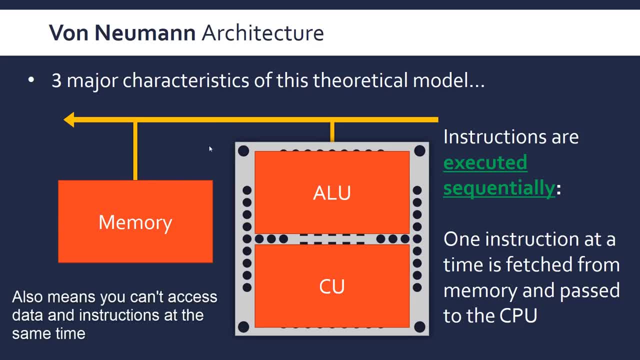 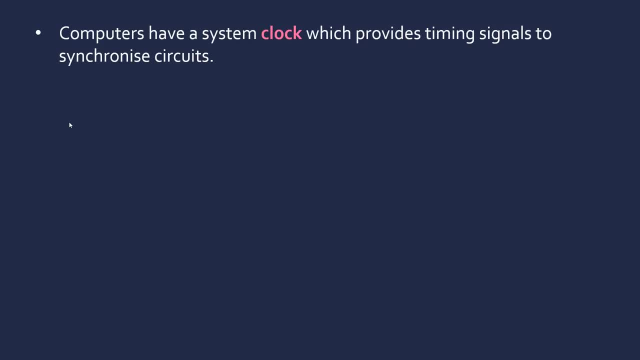 called a Von Neumann bottleneck, and that's just an interesting feature of this architecture. I mean, I say interesting anyway. um, we have to talk about the clock briefly in this topic. it's actually very important for the whole computer, but especially for the CPUs operation. so computers have a 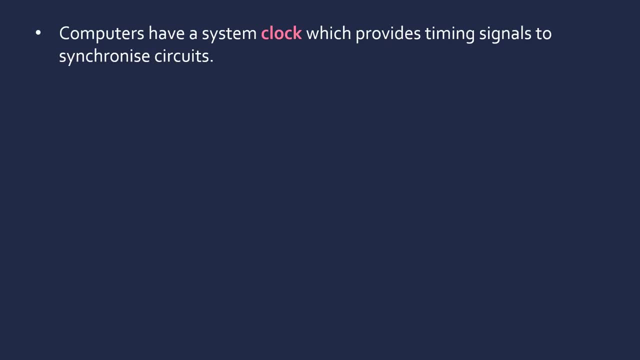 system clock which is actually there to provide just general timing signals. it's not specific to anything, it's just there to in the background. you can see that it's a clock and it's actually there to provide just general timing signals. it's not specific to anything, it's just there to in the background, to 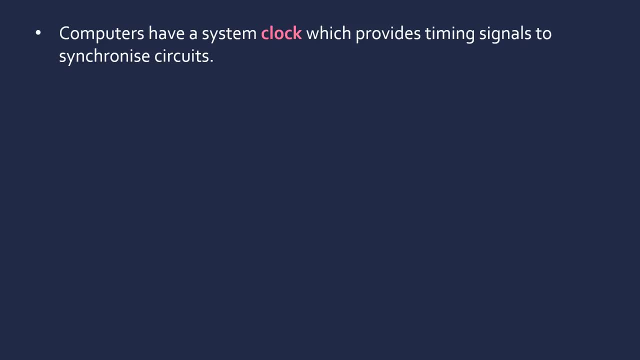 provide timely signals and it's used by the circuits- any circuit in the computer- to synchronize itself, and it's not like a clock, like we used to, it's like a metronome in music which kind of just produces a steady, steady rhythm, a steady pulse of voltage. this is representing two different voltage levels. 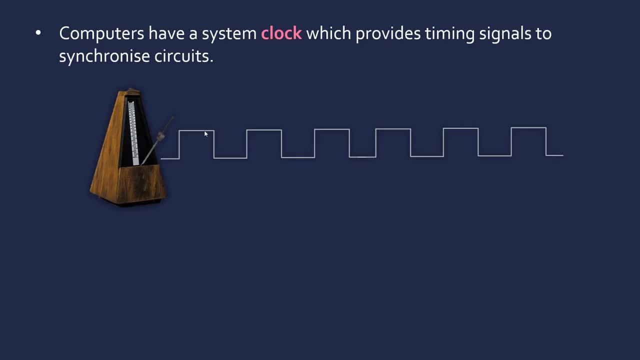 could be on and off, it could be five volts and ten volts, but the fact remains that it's a very steady kind of pulse, pulse pulse- and first of all, you can use it to synchronize your circuit. so, for example, you might only transfer data on a rising edge of the clock or you might only do on a falling edge of. 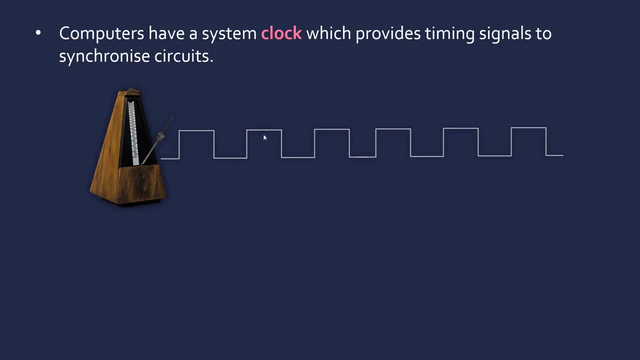 the clock. you might only write data when the clock is high, asserted high, or if it's asserted low. essentially, the devices can use the clock as they wish and the clock- the system clock, actually sits on motherboard and, like I say, it's used by any devices, but the CPU uses it and CPUs are designed and. 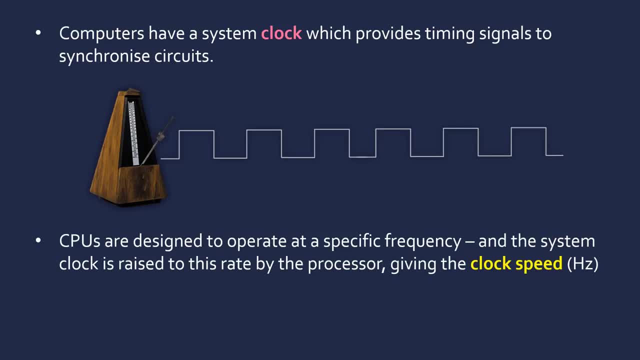 manufactured to operate at a specific frequency. the CPU is much faster than all the other components, so it needs to essentially have a clock that oscillates faster, that has a higher frequency, and so the CPU takes the system, clock and changes it so it's a lot faster, and this is the clock speed. 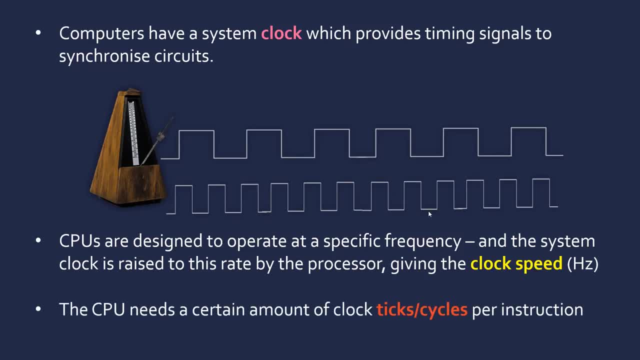 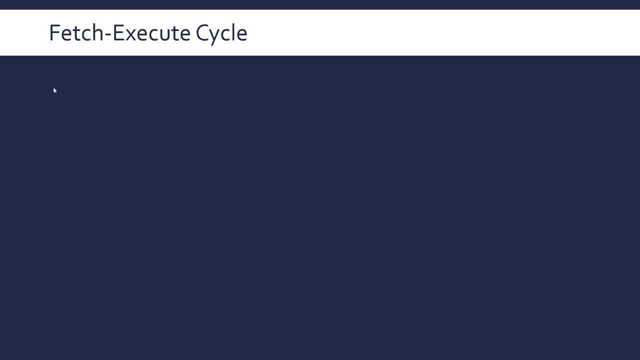 and the clock speed is very important because the CPU needs a certain amount of clock cycles or ticks, essentially an arbitrary amount of these. we could just say one, for example, per instruction. so it uses a cycle and this cycle is the fetch execute cycle. so all this does is this is just the 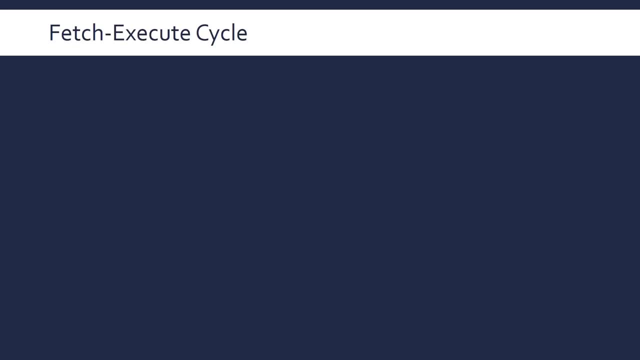 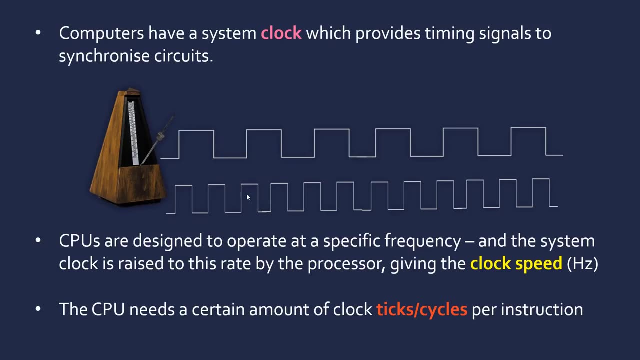 process of the CPU executing a single instruction. so if we just go back a second, it might execute instruction whenever the clock is high. so the instruction here, instruction here, instruction here and so on, and the faster this is done and the faster the CPU operate because it's got a higher 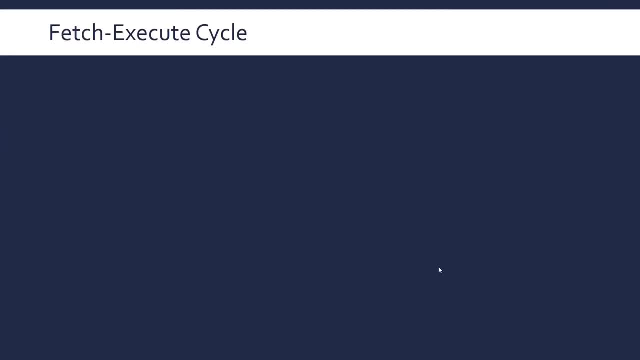 clock speed anyway. so the fetch execute cycle. first of all, as we've talked about this, the memory is external to the CPU and the instructions are stored in the memory. so they need to be retrieved by the CPU from the memory. and this is just a fetch stage of this cycle. so first of all, 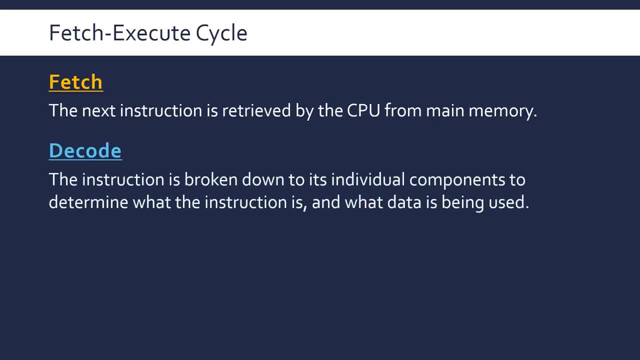 instructions go to the CPU. when they're there they go into the control unit and the instructions broken down into its kind of constituent parts, and an instruction is split up into its operator and its operand. the operator is telling you what it's doing like add in this example. 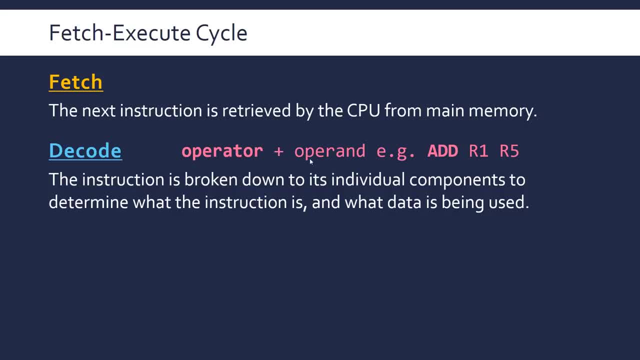 actually the addition here is an operator, and operand is another word for data, and so we have two operands here. these are two registers. so this instruction assembly code is saying we want to add the contents of our five register five to the contents of register one, and so in this stage it 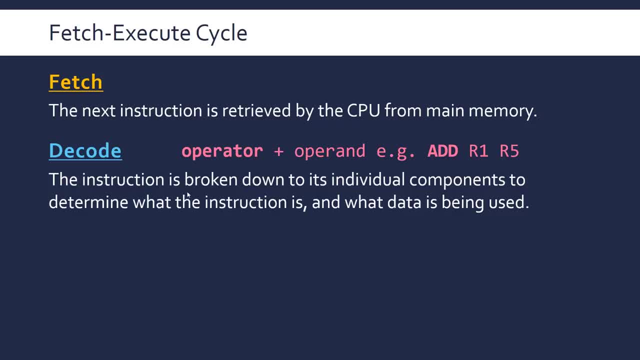 works and what the instruction is. depending on what the operator is, it will. essentially it's relevant for the execute stage, where the data is actually executed. here the CPU will use information that's got from the decoding stage to activate the necessary circuitry in the ALU, or if 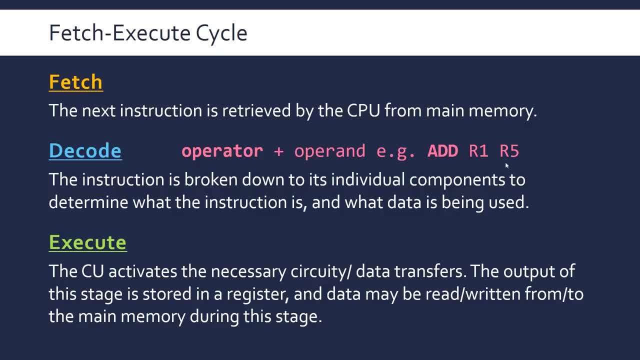 it needs more data, or if it needs to transfer to or from registers, like it does in this case, it will do it in the execute stage, and this is all done by the control unit, with the actual execution of the instructions for following of the instructions is done by the ALU, and the output of this is: